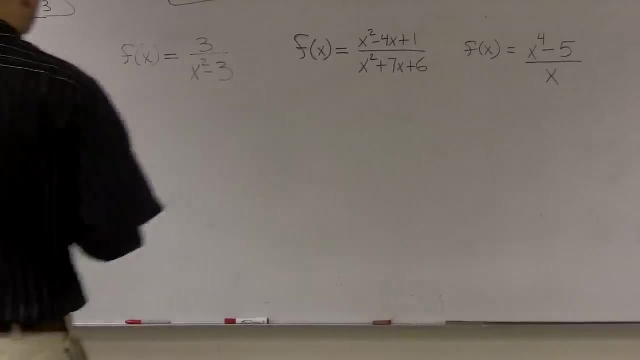 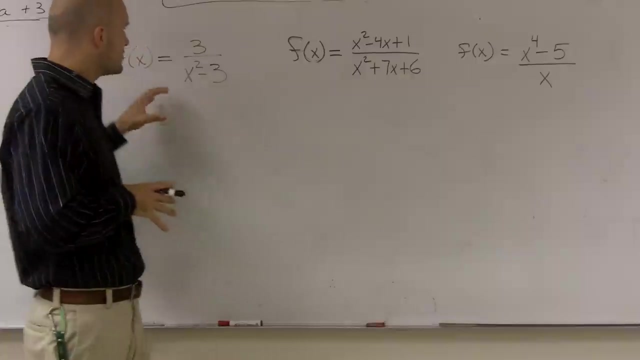 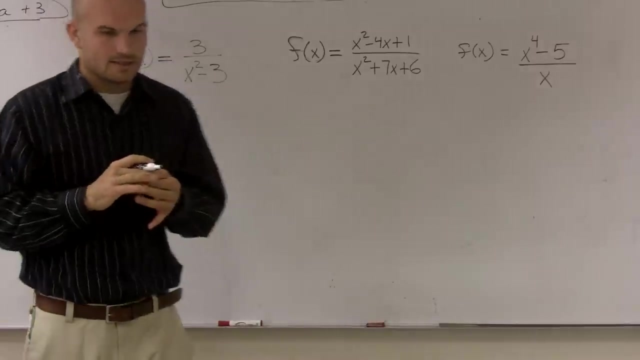 All right, what I'm going to do is I'm going to show you how to find the vertical and the horizontal asymptotes of a given function. So the first thing we want to do is when we're finding our vertical asymptote. our vertical asymptote is going to tell us pretty much. 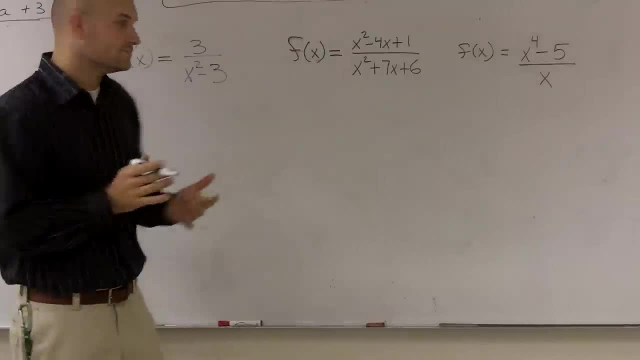 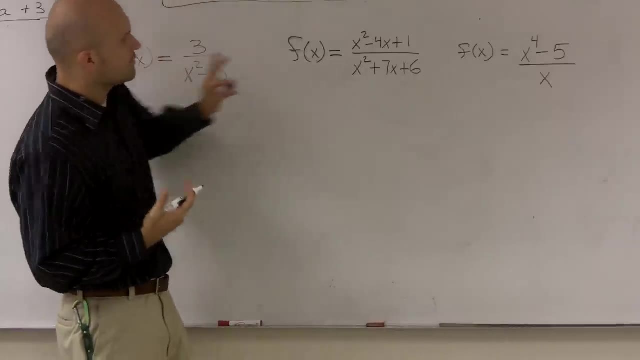 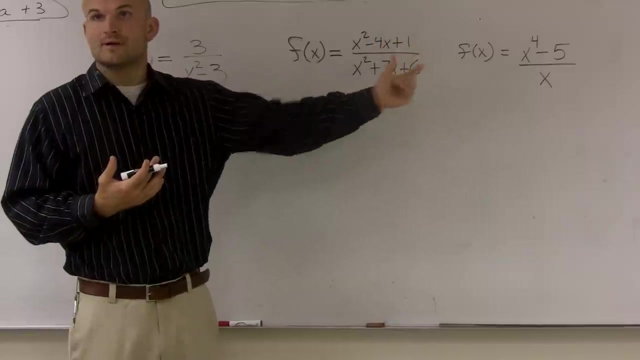 what values of our function are not going to cross on the x-axis. So what it's very similar to is actually finding the domain And if you remember, when you have a rational function to find the domain, you determine what values make it 0 on the bottom And whatever. 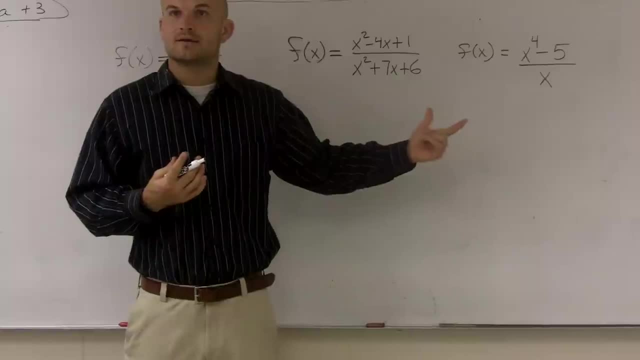 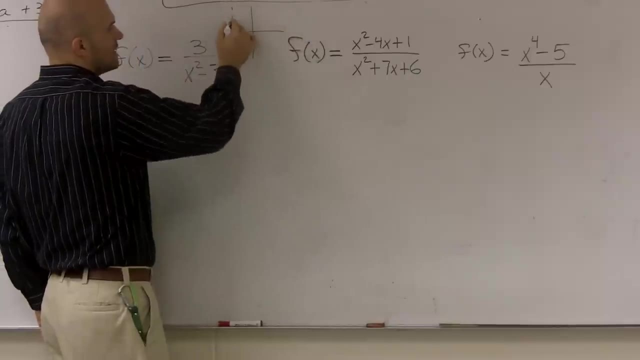 values make it 0 are not going to be a part of your domain. And that's the same thing with the vertical asymptote, Because if you think of a vertical asymptote, it's going to be a number, It's a vertical line that it's a value of x that your graph does not. 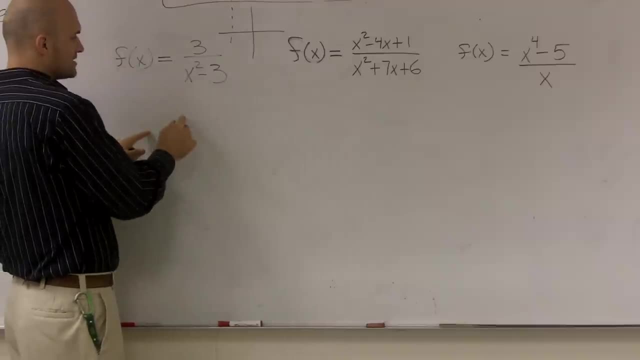 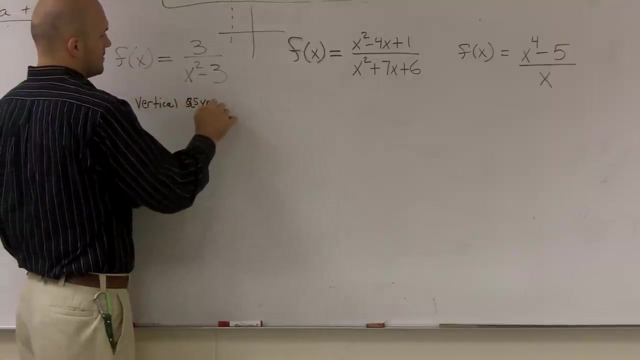 have or is not defined for. So to determine this, I'm going to set each one of my values. So when I want to find my vertical asymptote, what I'm going to do is I'm going to set the bottom equal to 0 for. 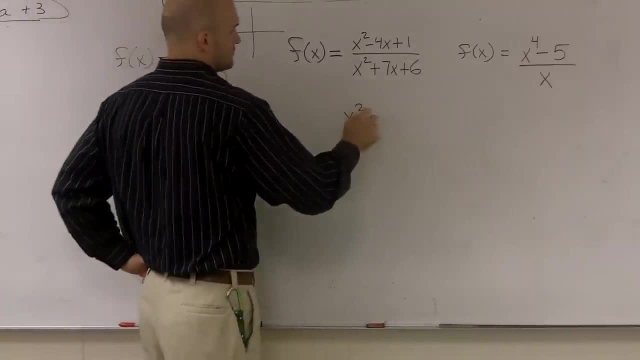 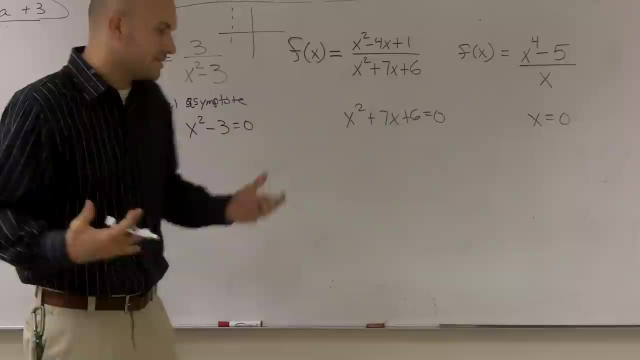 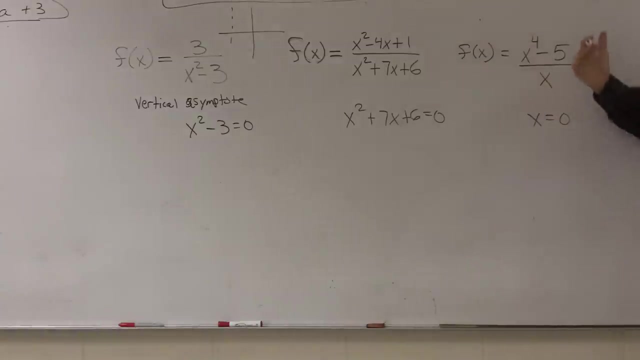 each problem, And this is just very similar to finding the domain. And the reason why is remember whatever values make it 0, that's not part of my domain. And since it's not part of my domain, it's not an x value in my function Or my function. 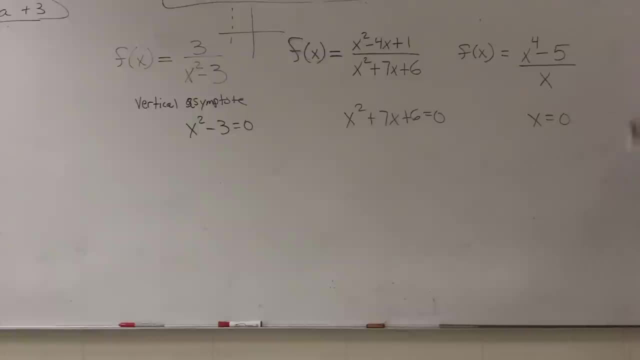 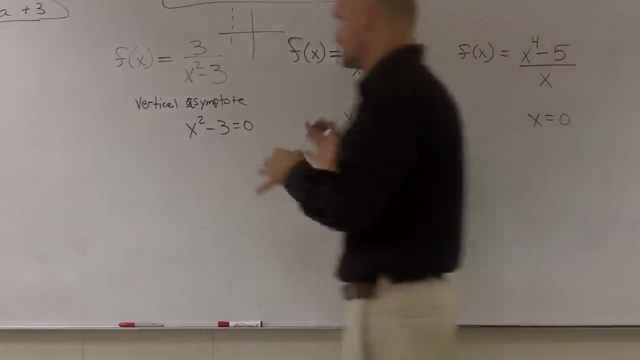 is not defined for that value. Therefore, it's called what we call an asymptote, And meaning an asymptote is when you look at a graph, the graph is never going to have a value at that point. And we'll get into it when we talk about graph And you guys 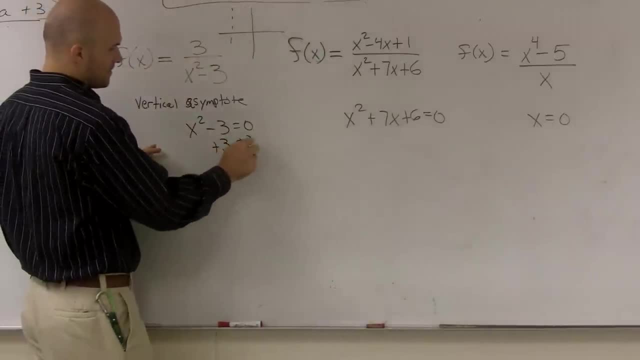 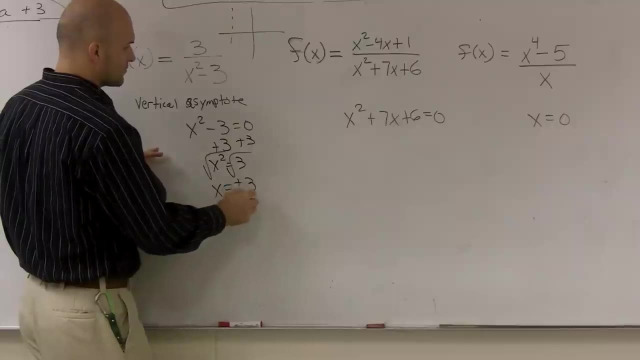 will see what I'm talking about. So here I'm just going to add 3. x squared equals 3.. Square root x equals plus or minus Square root. Square root 3.. I'm sorry, Square root of 3.. 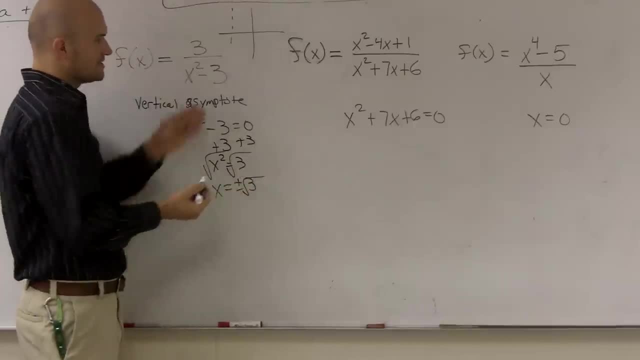 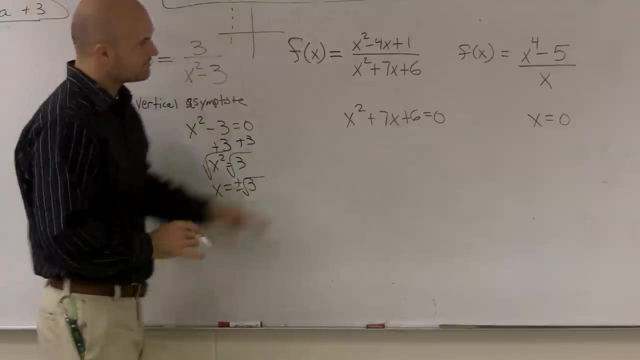 Yeah, Right. So therefore my vertical asymptote for this problem, that means the x values are: x equals plus or minus the square root of 3.. So we'll get into graphing later Here to find the vertical asymptotes. I set it equal to 0.. And here, since I have a trinomial, 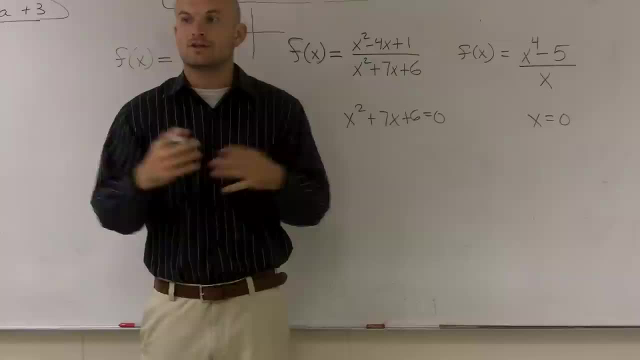 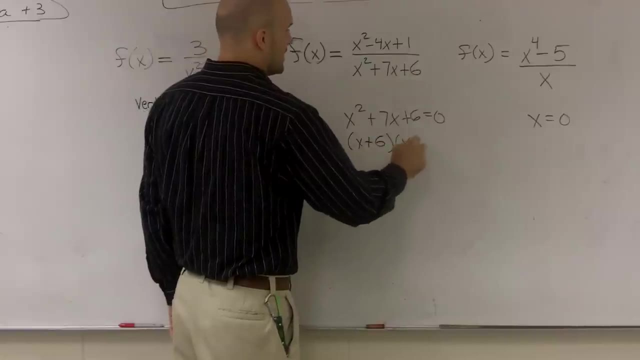 I can't do adding to the other side. When I have a trinomial, I'm going to look for factoring And I see that this can be easily factored into x plus sin. So x is 0.. That's because y is negative. 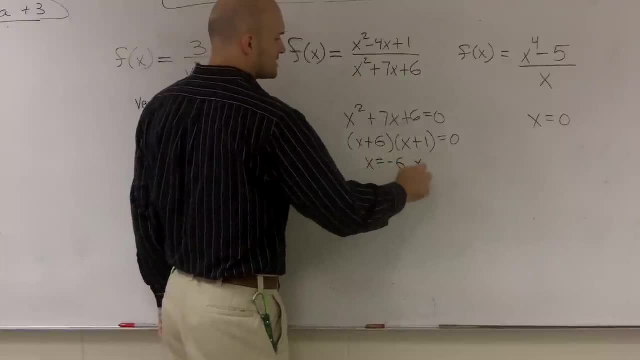 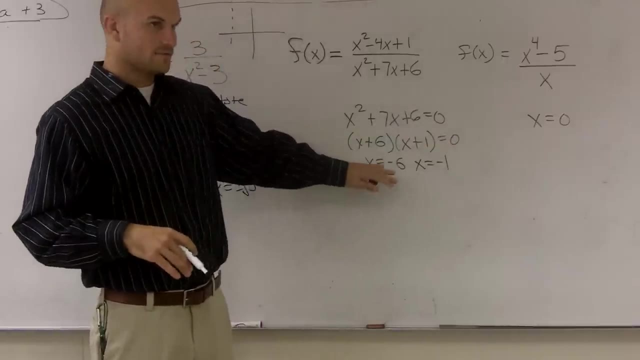 Now, what do I? What do I do? So I'm going to do a 1i-sqrt, or I try to do a, a frivolous molecule, And this is from the fundamental Theres leaf. So lets do a exponential, Small total of 6.. 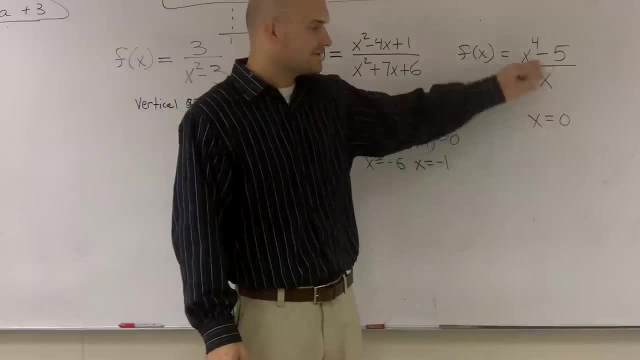 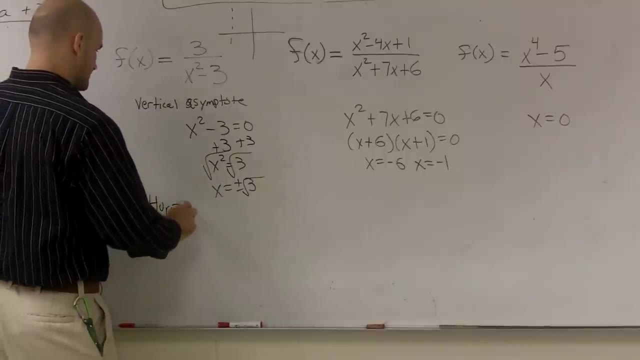 And x plus 1, equals 0.. Therefore, my asymptotes are: x equals negative 6, and x equals negative 1.. So I'm just going to make it a little quicker. Remember, just set each of those equally to 0, and then you solve. 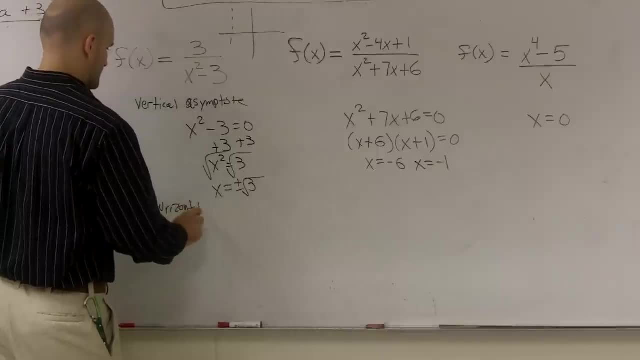 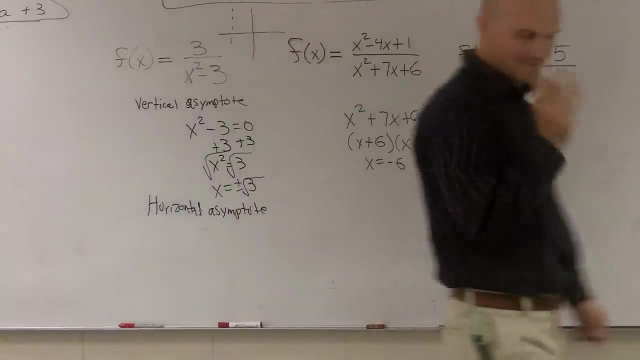 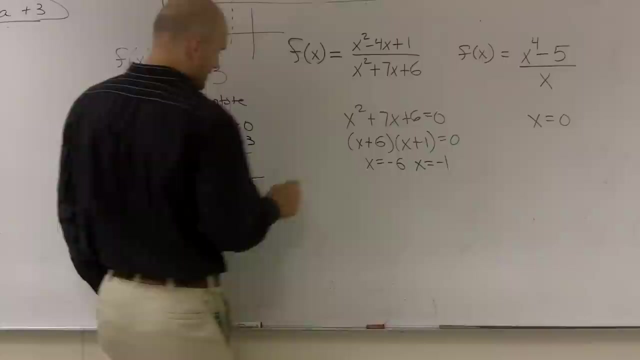 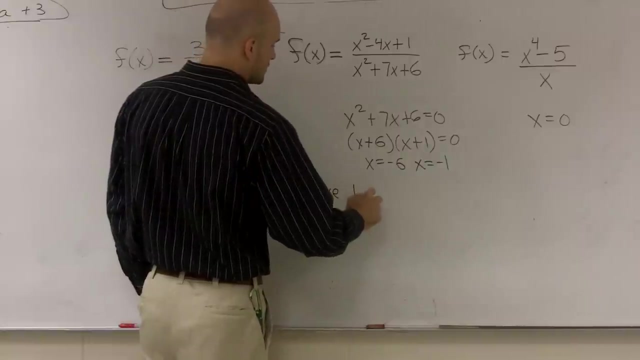 Right, OK, Here, this one's very easy. So when you want to find your horizontal asymptote, what we need to do is we're going to look at. there's two things. we need to look at our leading coefficient, so we need to compare. 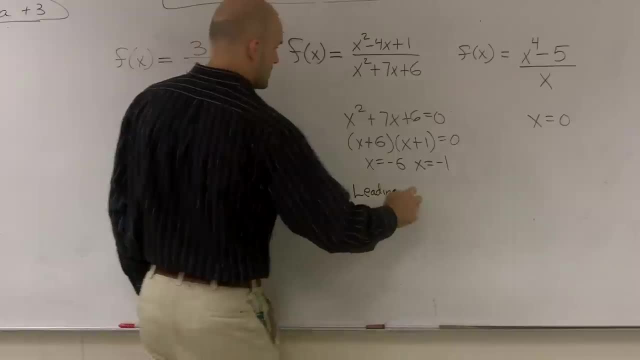 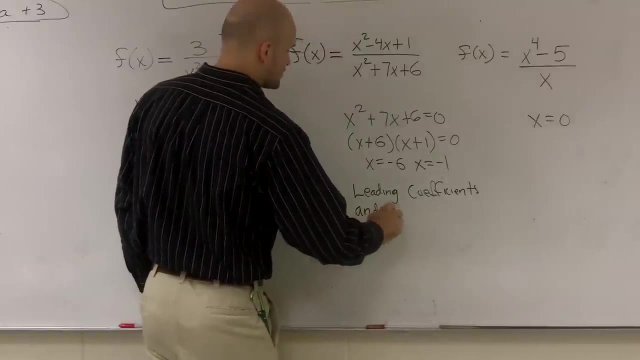 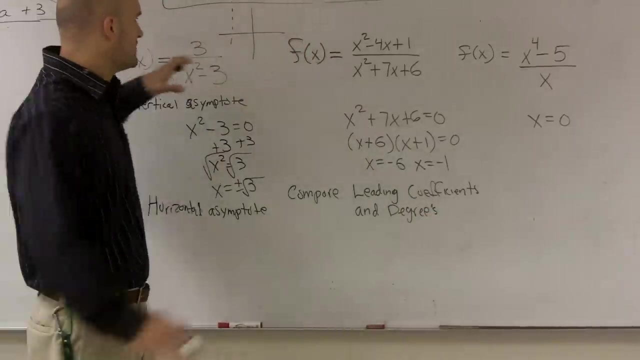 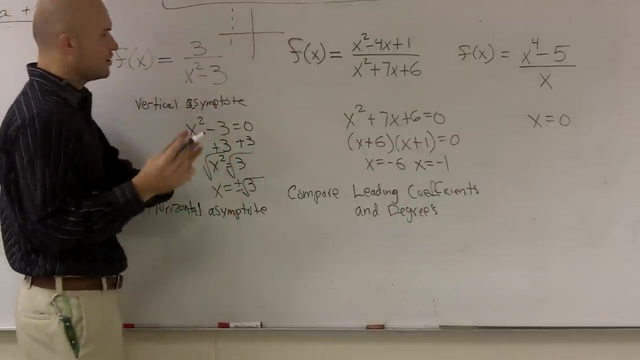 our leading coefficients and degrees. So when you guys look at each one of these problems, we need to look at the leading coefficient and the degree of our leading term. So here of each polynomial, so at the top and on the bottom, So we're going to compare leading coefficient and degrees. 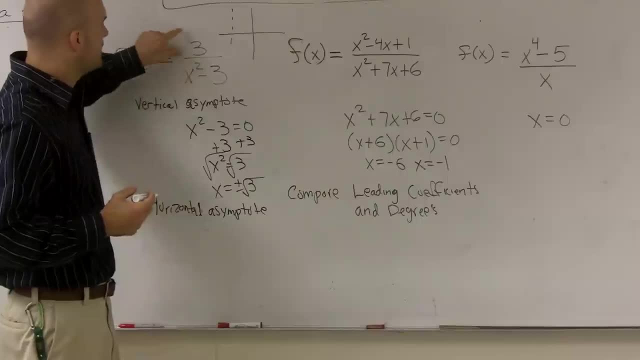 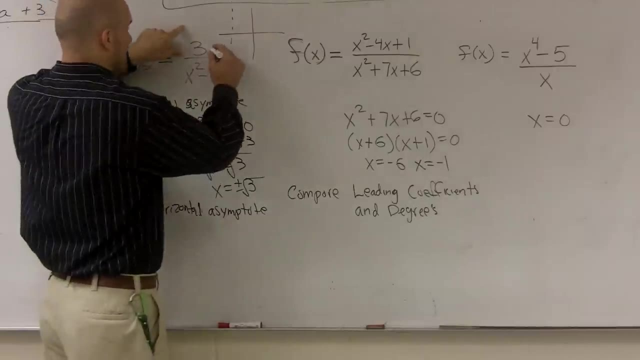 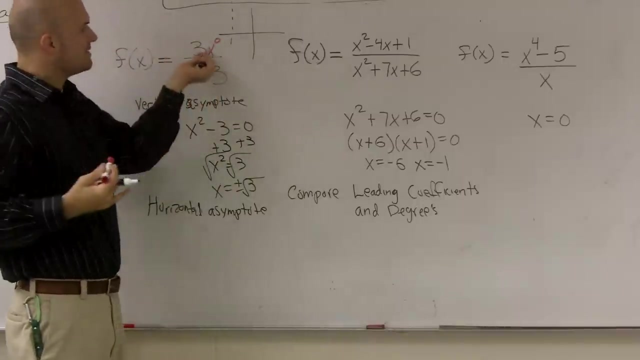 For your polynomial up top and polynomial at the bottom. Here we have a polynomial, but it's a constant polynomial. Now a lot of you might say, well, there's no x right there. right, Well, I can. I can put x to the zero power, because any number raised, anything raised, 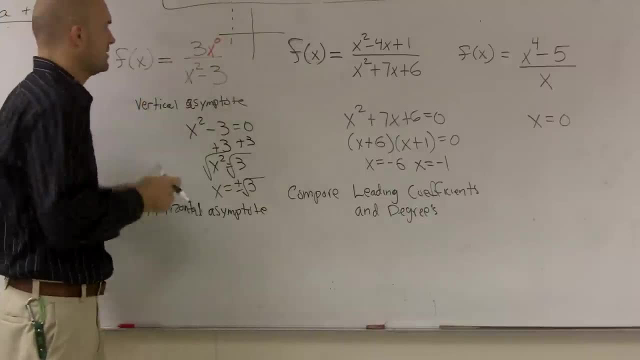 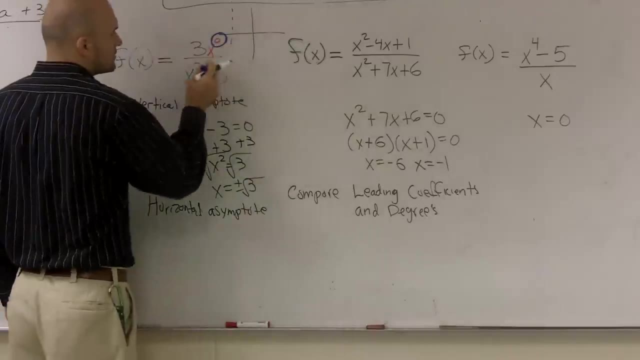 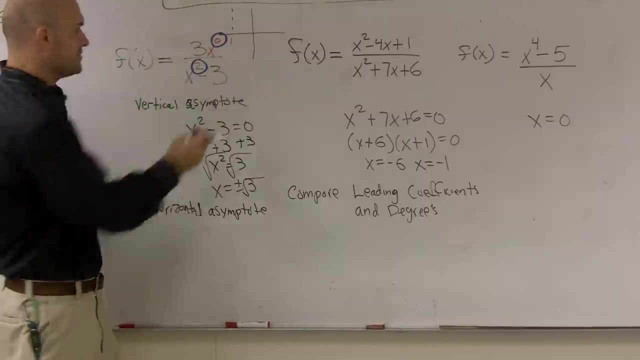 to the zero. power equals one right. One times three would be three. So then the next thing I want to do is I want to compare my degrees. Alright, And when my degree up top is less than the bottom, so when zero is less than two, the 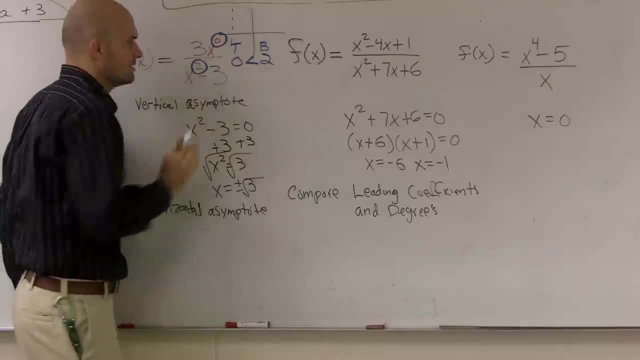 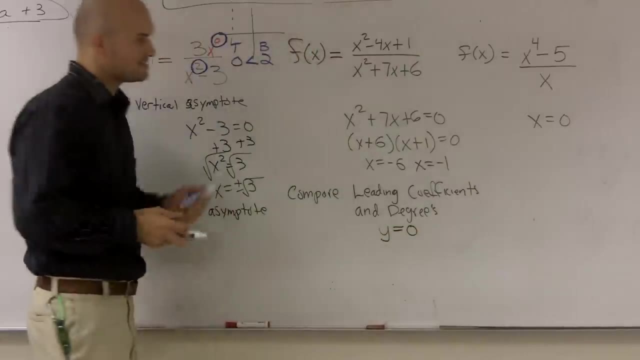 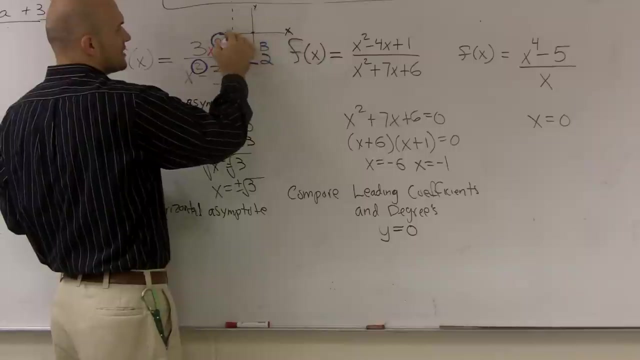 top is less than the bottom right of your degrees, my horizontal asymptote is going to be: y equals zero. And I'm saying y because you know this is your y axis and that's your x axis, So my y values can equal zero. 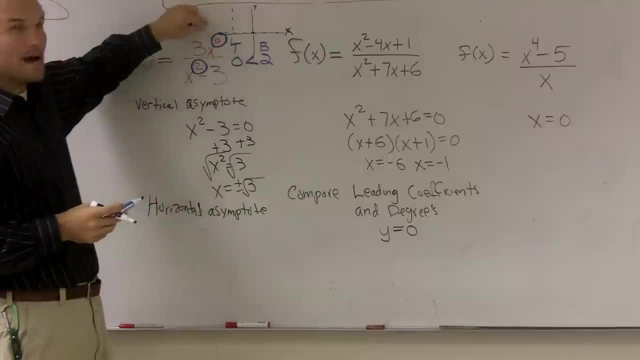 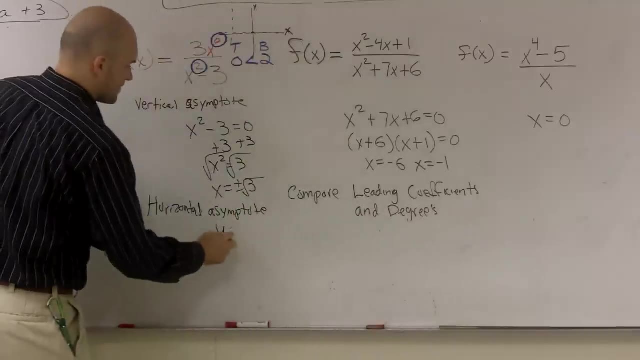 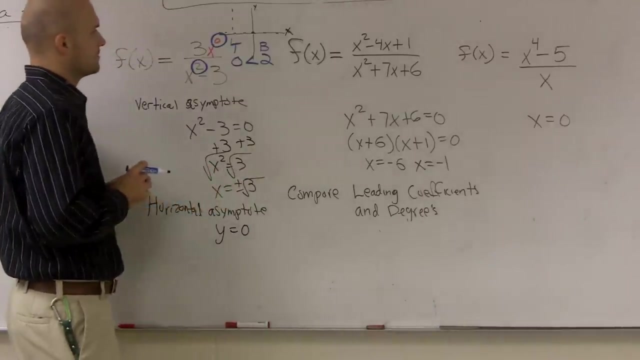 Alright, Zero. So whenever your top degree is less than your bottom degree, your leading coefficient- I'm going to do that over there- y is equal to zero. Okay, Next one. What Is that? because you divided zero by two. 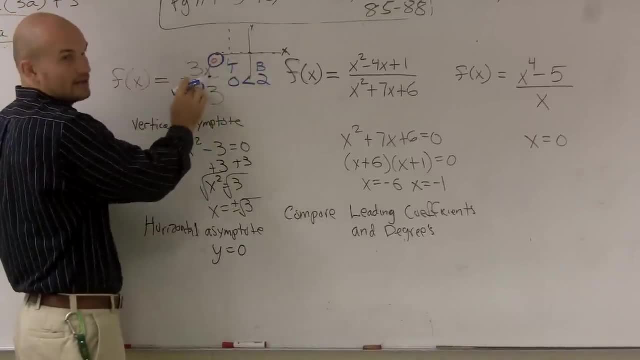 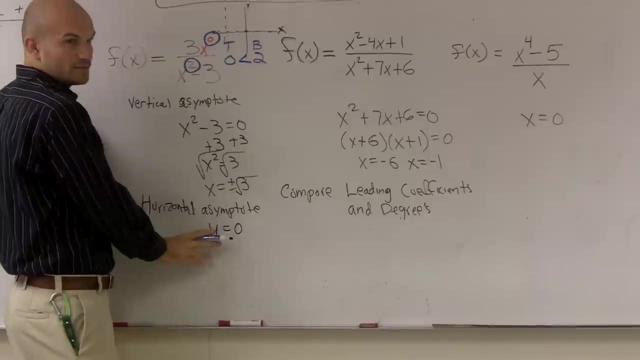 No, It's just whatever. It doesn't matter if that was one and that was three. Whenever you have a top is large, is smaller than your bottom degree, it's always just: y equals zero, Always. It doesn't matter if it's five and fifty. 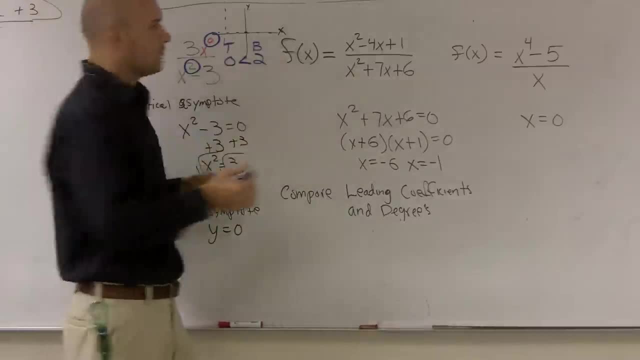 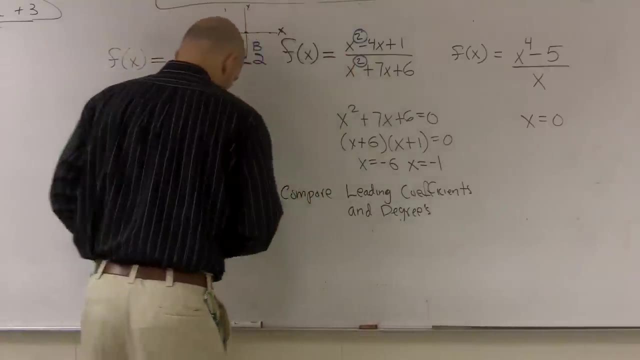 It's less than zero, it's less than so y equals zero. Now, when you have that equal, okay, what you do is you take the number in front, which. there's no number in front here, right, So we write one. 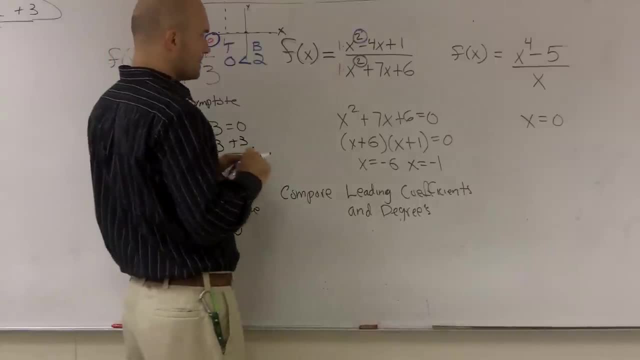 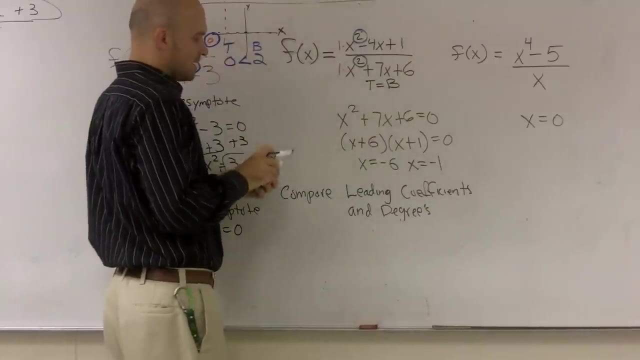 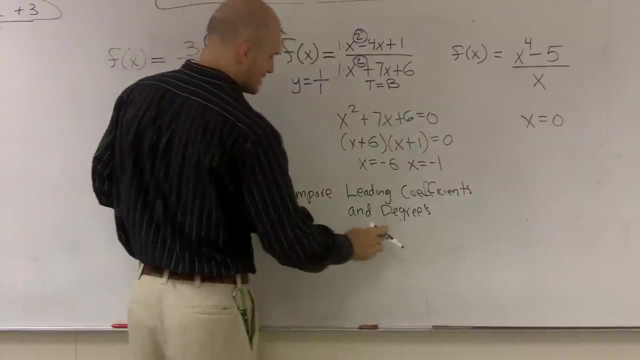 You take the number in front and you divide them. So whenever they're equal, so when you say like the top is equal to the bottom, what we do is we take our coefficients and we divide them. So we say y equals one over one, which is one in this case. 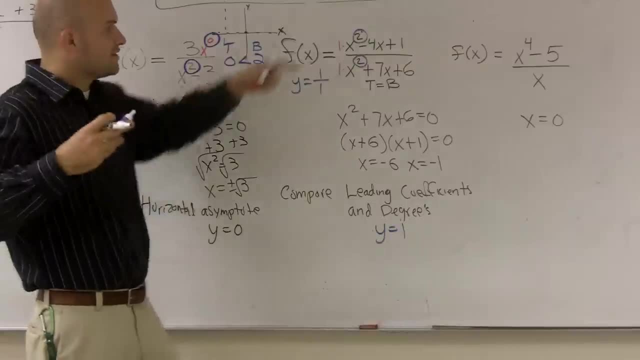 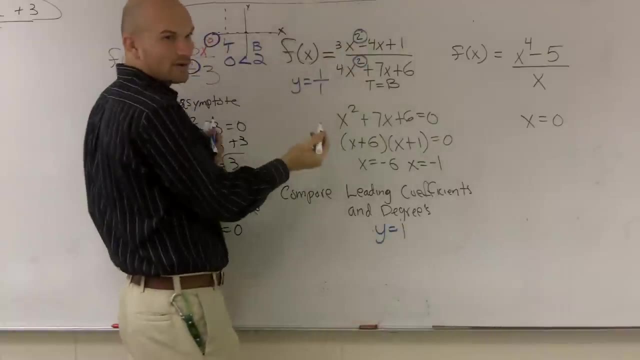 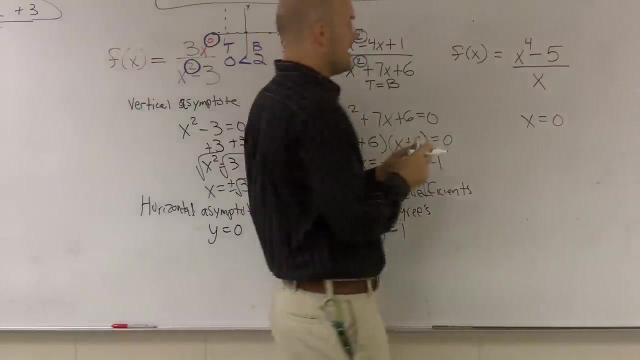 Does that make sense? So whenever they're equal. so if this was like, if this was like a three-fourths, then it'd be three-fourths, right? So just always divide the coefficients And then now, when we have, we can put a one there. 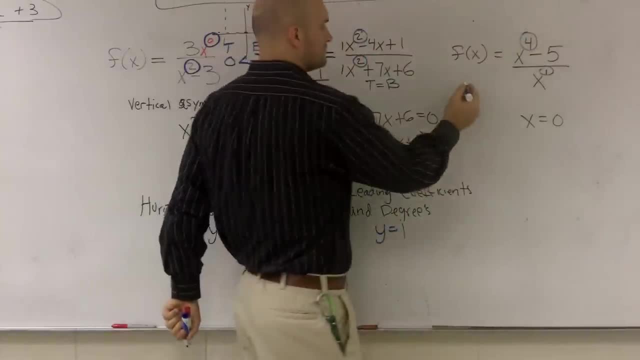 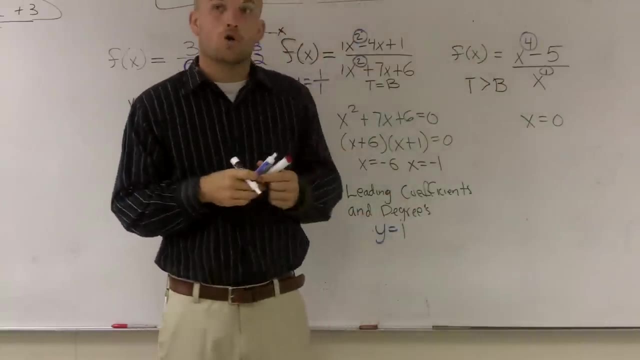 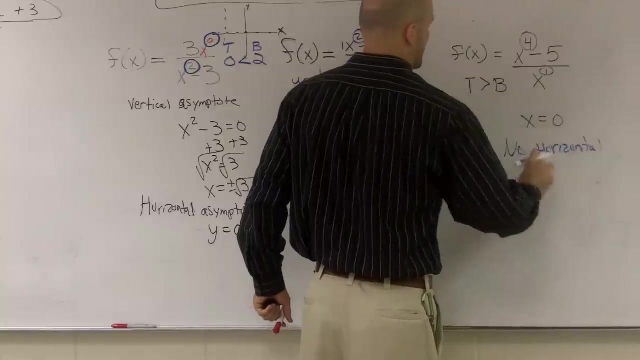 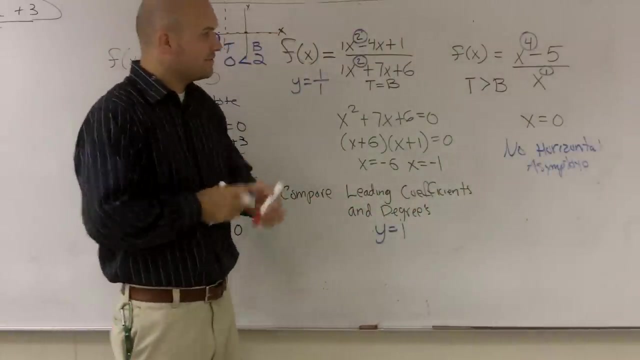 Whenever we have, the top is larger than the bottom. so you can say: the top is larger than the bottom. we- there is no horizontal asymptote, No horizontal asymptote, And we will. that means there's going to be a slant which we'll show in another video.